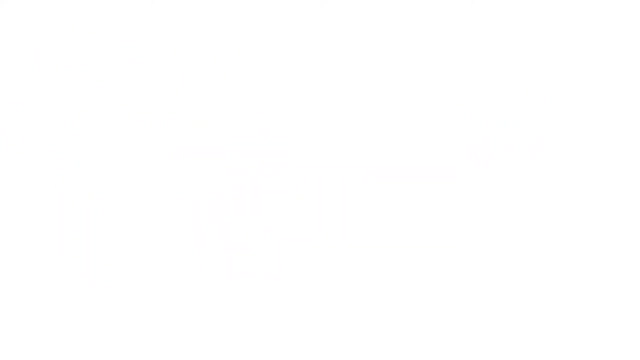 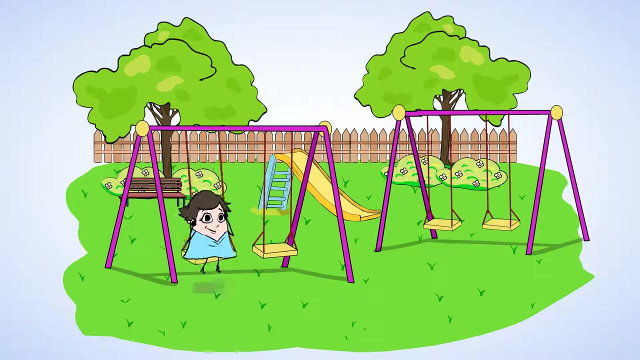 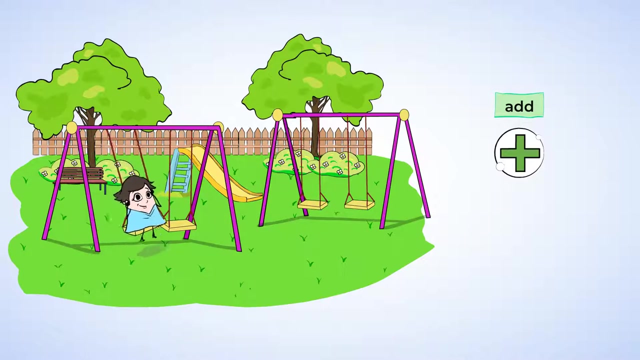 Hello, this is Mighty Owl. Look, it's Mia. She's in the park today on the swings waiting for her friend Jenny. They agreed to meet us and help us learn how to add, But right now Mia is at the park alone. 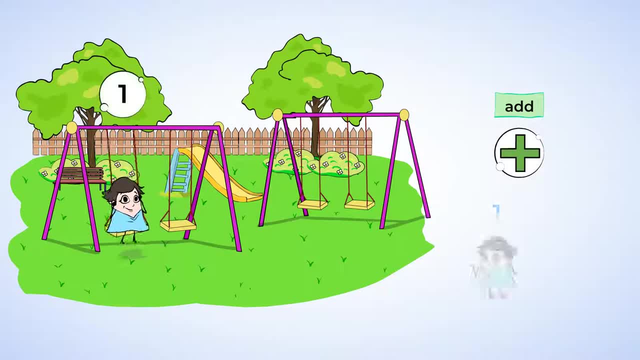 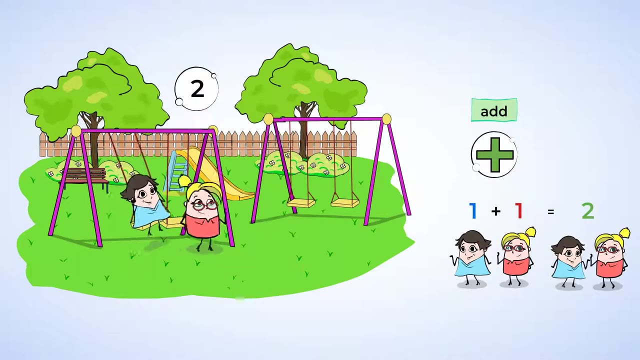 And if she's alone, well, that means there's only one person at the park. Oh, but here's Jenny now. Hi, Jenny, And now that Jenny is here, there's one more person at the park, And so there are two people at the park all together, Mia and Jenny. And you know what we? 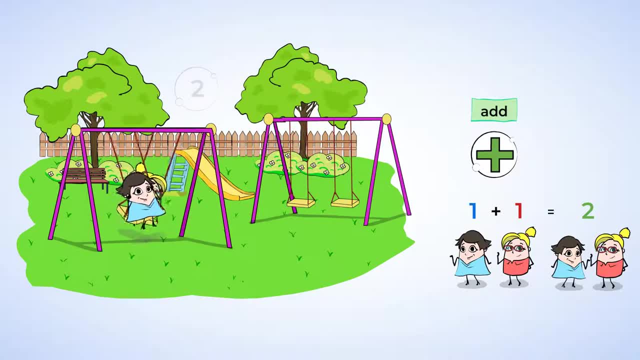 just did. We just added two numbers. Addition is when you put things together to make a bigger number. We put one person and one person together for a total of two people. The total, that's how many things or people in this case, you have in all. Great job. Wow, it looks like Mia. 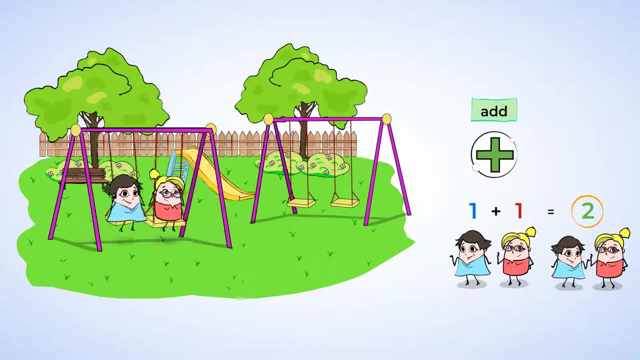 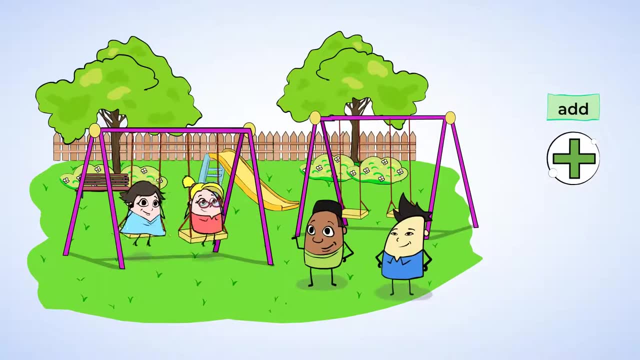 and Jenny are having such a fun time on the swings- Look at how high they're going. And more friends are arriving. Will and Chen are coming to the park to play as well. First we just had two friends in the park, Mia and Jenny, And now we have two more friends, Will and Chen. Do you think? 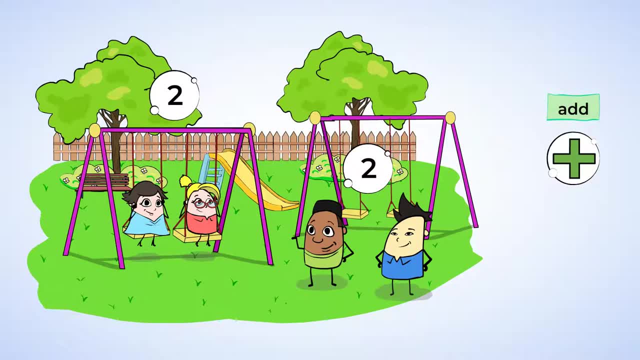 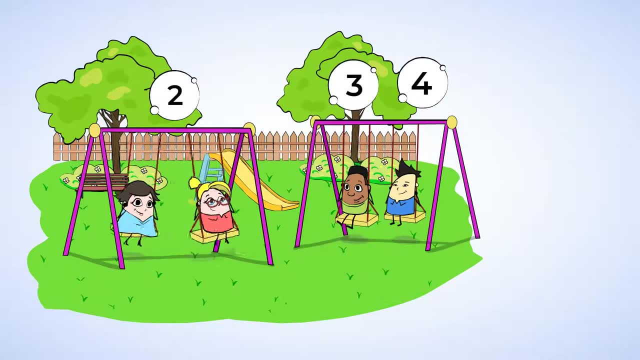 we could count all of the friends. Yes, we could. We can start from two and count up Three, four. There are four friends in the park. Wow, Now all four friends are swinging high on the swings. And look around them. Do you see those cute bunnies? 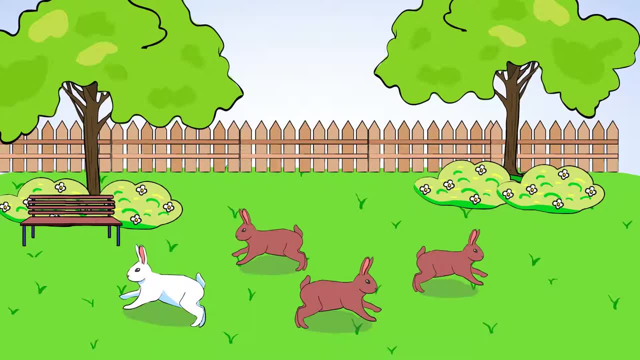 hopping around in the grass. Aw, they're real cute. How many white bunnies do you see? Just one. There is one white bunny, And how many brown bunnies do you see? Well, let's count them together. 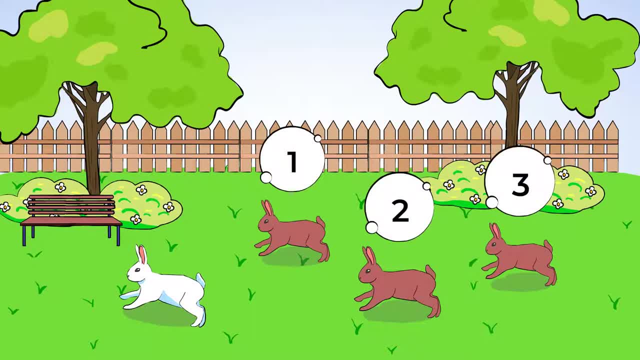 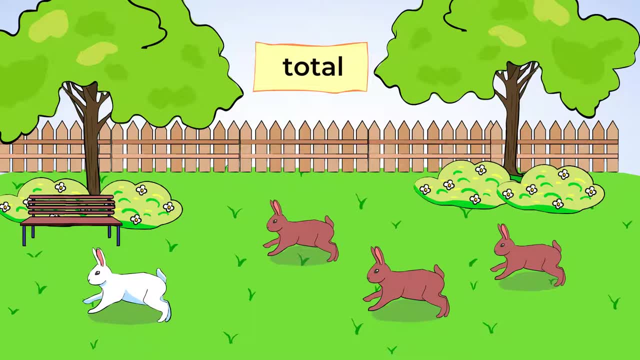 One, two, three. There are three brown bunnies in the field, But how many bunnies are there in total? Total, remember? that means all of the bunnies together. Well, to find the total number of bunnies, we can put these two groups of bunnies together. We can add one bunny to the other three. 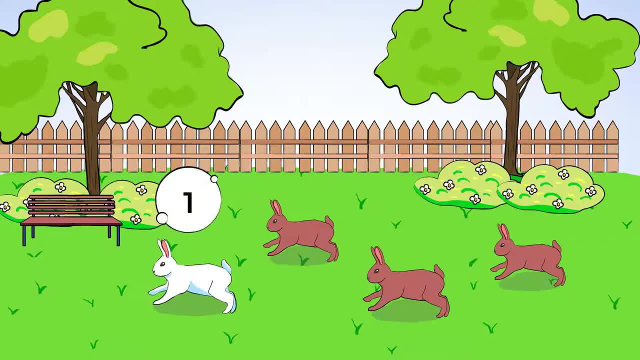 bunnies and count them together: One, two, three, four. We can also take the three bunnies and add the one bunny and count Three, four bunnies. We can actually count, starting at any number, And either way there are four bunnies all together. Great. 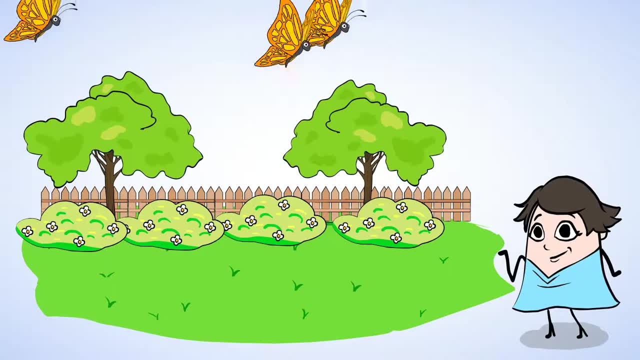 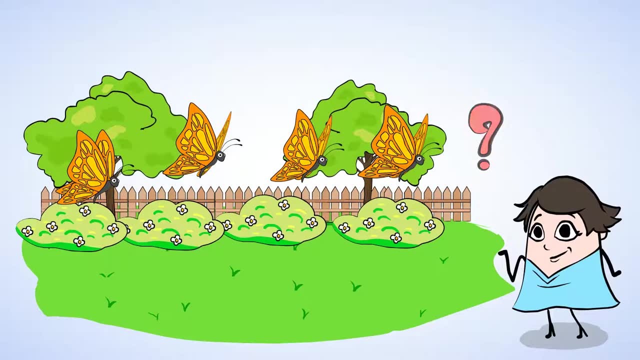 job. Wow, what a beautiful day. Look, some butterflies have flown into the playground. I wonder how many butterflies are there in the playground? Well, let's count again: One, two, three, four. There are four butterflies at the playground And here come two more butterflies. 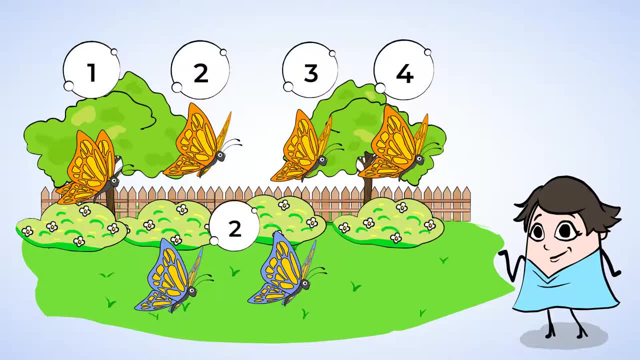 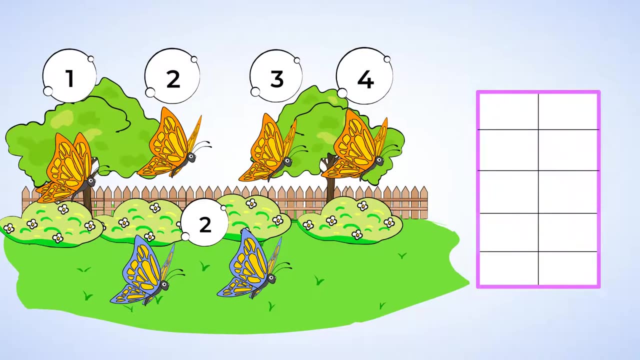 Well, first we had four butterflies And now we have two more butterflies, So we can add to find how many butterflies we have in all. Sometimes it isn't as easy to count the objects we're adding, But don't worry, There are many other things to help you add. Let's draw a picture to help us. 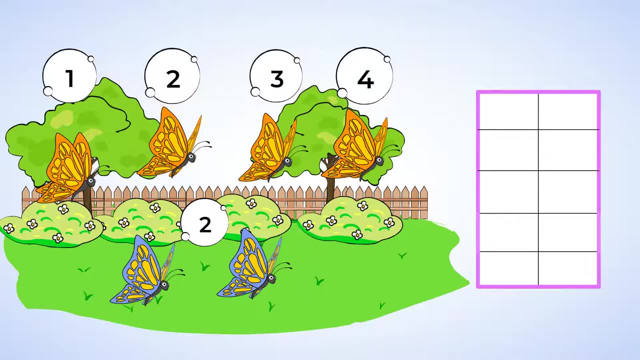 First we had four butterflies, right. So draw four butterflies: One, two, three, four. And now we want to add two more butterflies. So we're going to draw two butterflies, One, two, Now to add four and two. we count all of the. 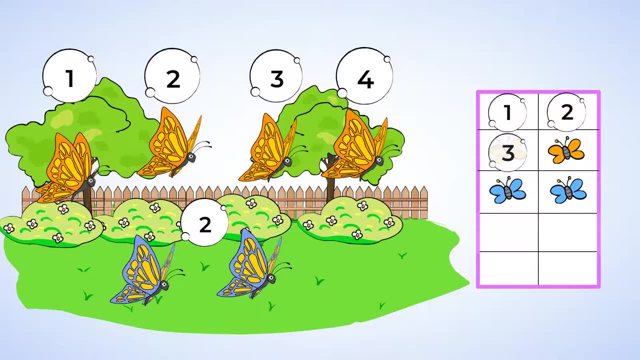 butterflies you already drew: One, two, three, four, five, six. There are six butterflies in all. The total number of butterflies is six And we can count the actual butterflies to check. One, two, three, four, five, six. Amazing, We were. 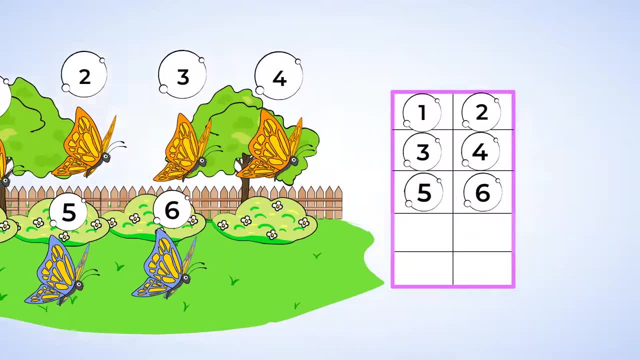 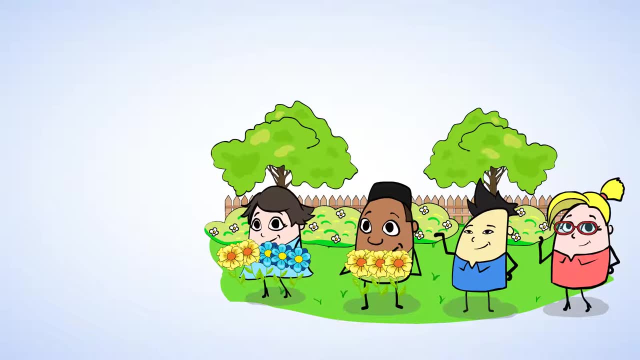 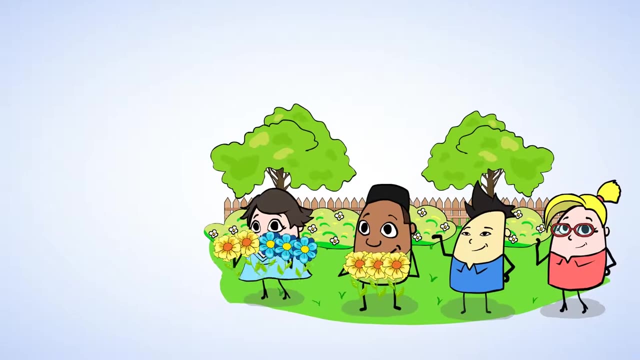 right, There are six butterflies in total. Oh and look, our friends are back. Mia, Jenny Will and Chen took a walk in the park and collected some flowers along the way. Oh, they sure are beautiful. Look at Mia's flowers. 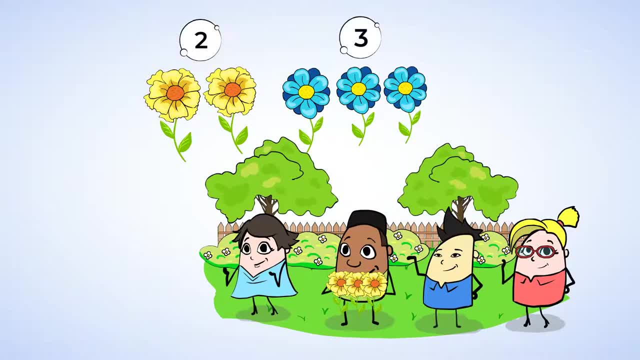 Mia has two yellow flowers and three blue flowers. Well, we can add two and three to find out how many flowers Mia has in all. Last time we drew pictures to figure out how to add. This time let's use our fingers. Yeah, that's right, You can count on your fingers to help you add. Now here's the number two.